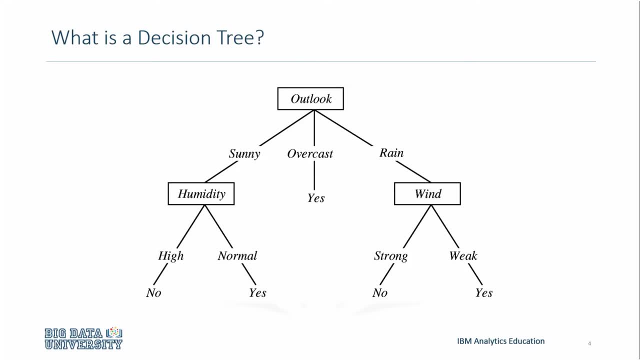 of the data. These categories can be called subsets, With the data set divided. inputted out-of-sample data will be classified more easily when it falls into a node that is strictly one subset of the data. If so, there's a higher probability that the data point 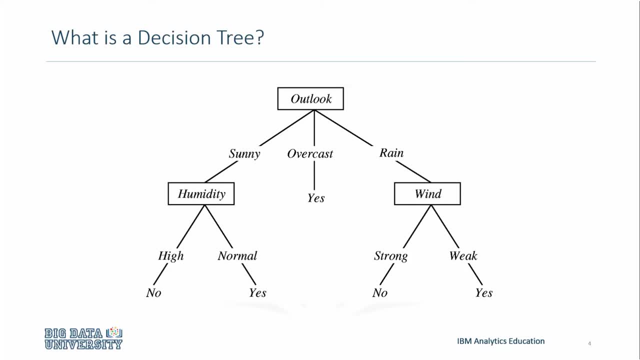 is the same classification as the node it fell under. So if we look at the diagram here, we can see that it's a weather classifier. So to make this more interesting, let's say that we want to go out for a run, but the decision to go out will be influenced by the weather forecast. 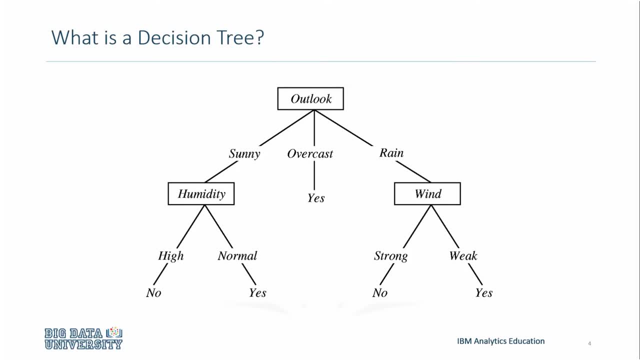 We start with the outlook, which can be sunny, overcast or raining. Our preference is to run on an overcast day. We can also run on a sunny day. We can also run on a rainy day. So if the forecast says it's going to be overcast, then we'll definitely go out for. 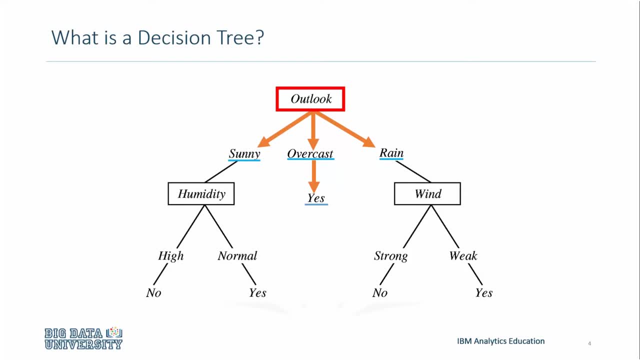 the run. On the other hand, if it's sunny or raining, we'll need more details to help us determine if we want to go out running. The additional forecast variables can be things such as humidity, wind and rain, For example, if the forecast is calling for high humidity. 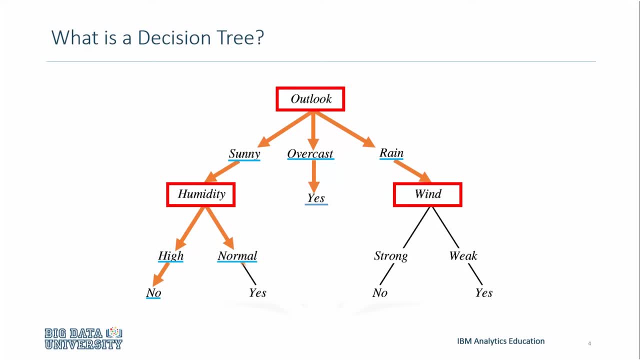 then we're not going on our run, but if it's normal, then we are. Similarly, with the wind on a rainy day, If it's a strong wind, then we're definitely not going, But if there's only going to be a 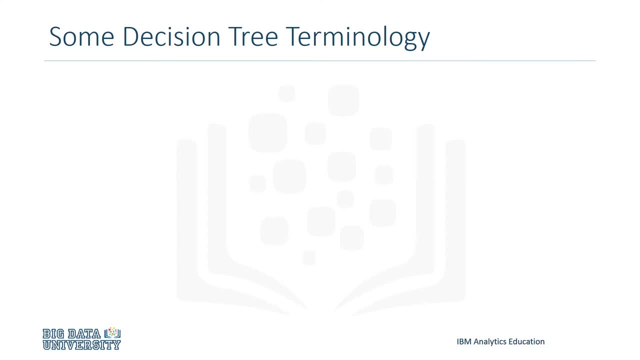 slight breeze. then we are Next. let's quickly review some terminology that can apply to decision trees. If some of these definitions don't make sense right now, don't worry, as we'll be going through some examples that will clarify this. First, we have a node. In a node, we have a. 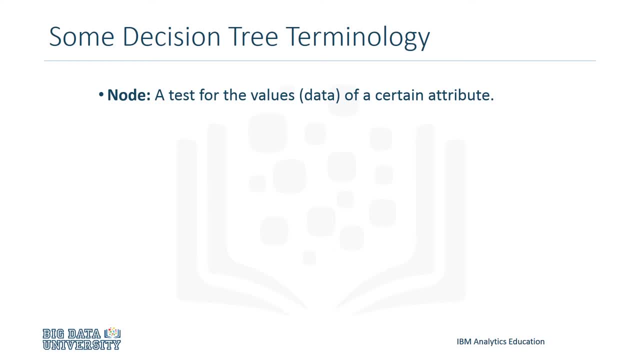 dataset that gets tested for a certain attribute. The goal of the node is to split the dataset on the actual tree with the level of the data, browsing volume or forecast value by tracking Rs. The goal is to get the viewing dept of Admin scores that depens from an identity. 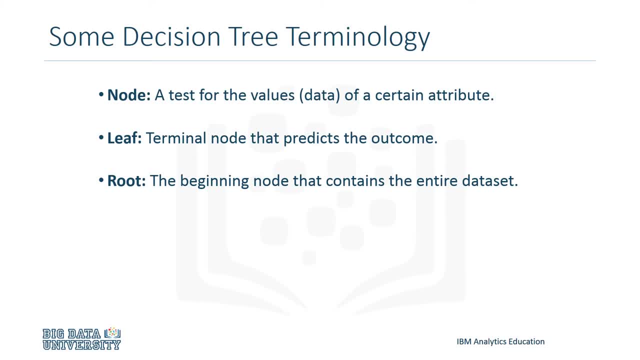 data. In some cases it's almost impossible to track the viewing data. if the data in is up to average to what the desired ratinguczeker set said was at agein 2.. Among Here you see the yellow blue. This is for each of these. 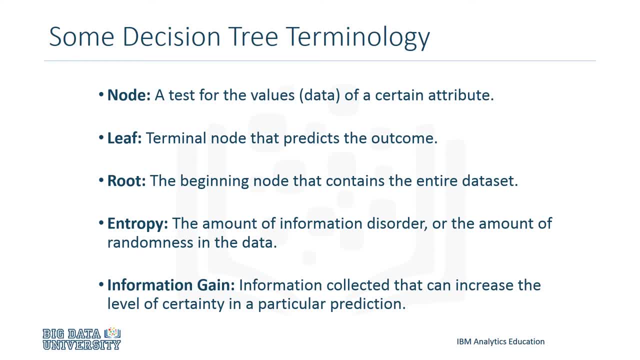 Next we have information gain. This is the information collected that can increase the level of certainty in a particular prediction. We can think of information gain and entropy as opposites: As entropy or the amount of randomness decreases, the information gain or amount of certainty increases, and vice versa. 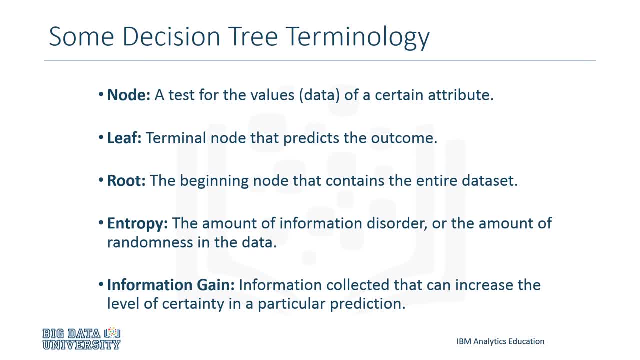 There are also mathematical formulas that you can use to calculate the entropy and information gain in each node to ensure you've made the best split. However, examining those formulas is outside the scope of this lesson. Let's take a more in-depth look at entropy and information gain. 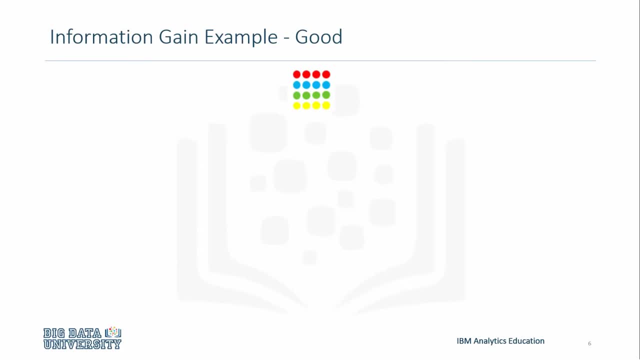 Here we have our data set at the root node, consisting of four colors: red, blue, green and yellow. There are four dots for each color, totaling 16 dots. We'll be using histograms to look at the chance that an out-of-sample data point would be a certain color. 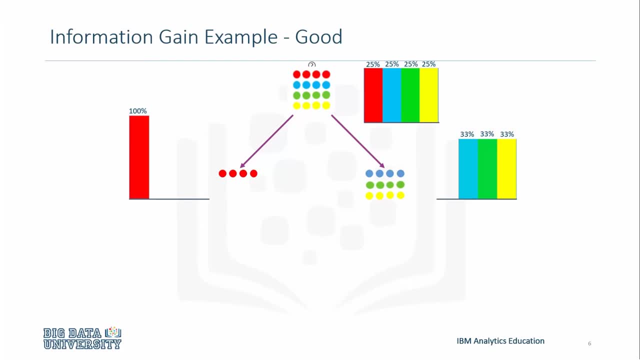 So we start off having a look at the data set. We start off having an equal chance of 25% for all colors. Let's say we make a binary split on the node. Note that in these examples the attribute used in the split will be ignored for simplification. 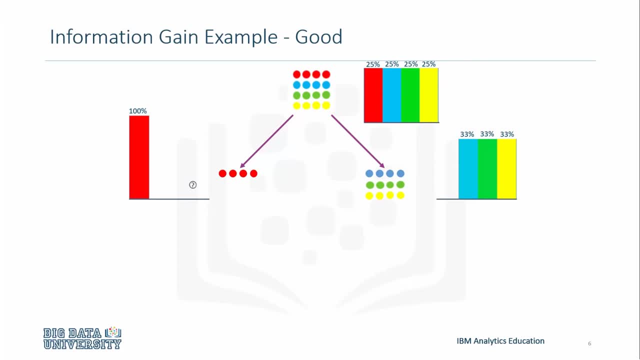 From this split, all of the red dots go to the left side and the rest of the dots go to the right side. Now let's take a look at what the histogram looks like for this split. A split that looks like this is ideal. 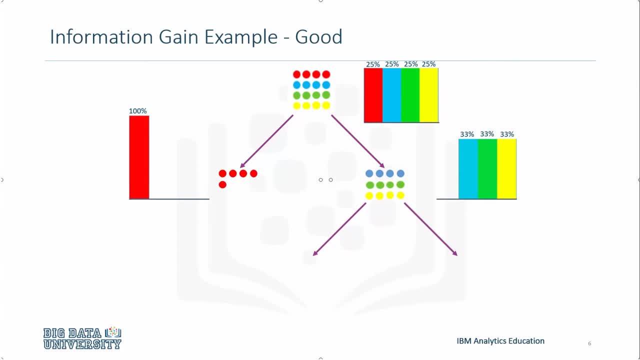 This would produce the most information gain and greatly decrease the entropy. Let's say we just take a look at the histogram. Let's say we stopped here and we wanted to put an out-of-sample point into our tree. We'll want to decide what color this point is. 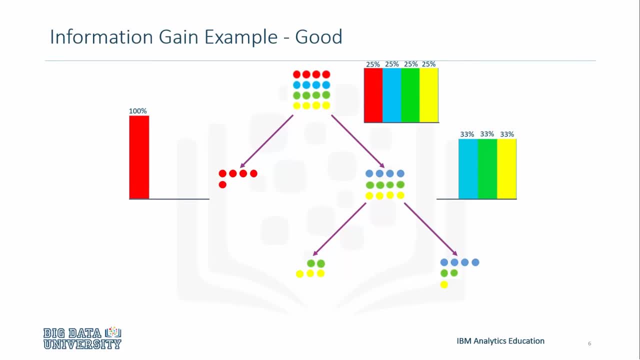 Let's say that this point fulfills the condition to be on the left-hand side. We can most likely say that this point should be red. Now back to the tree. The split we saw here is the best-case scenario. Most likely, though, we'd see a split that would look like this: 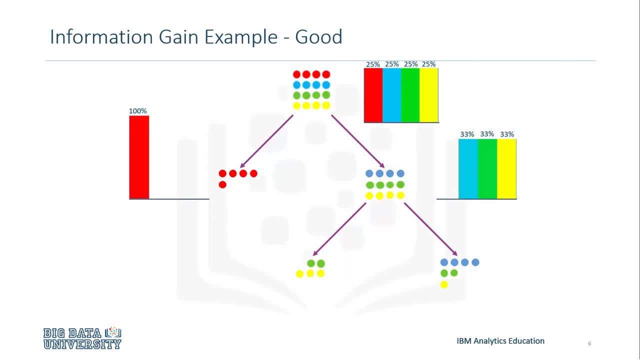 We can see that the split isn't perfect, but the right split has the highest chance of being blue, But it's not 100% like the first split with red. Let's also look at the histogram for this split. And now let's throw in another out-of-sample point.